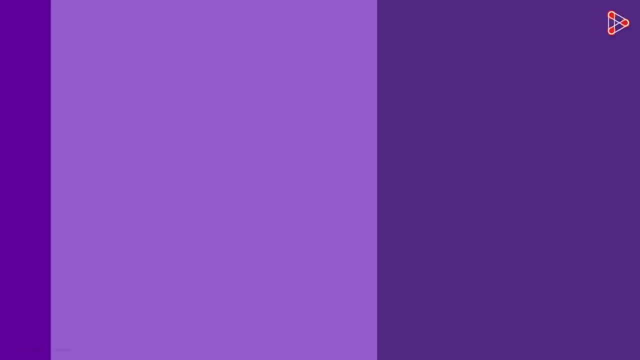 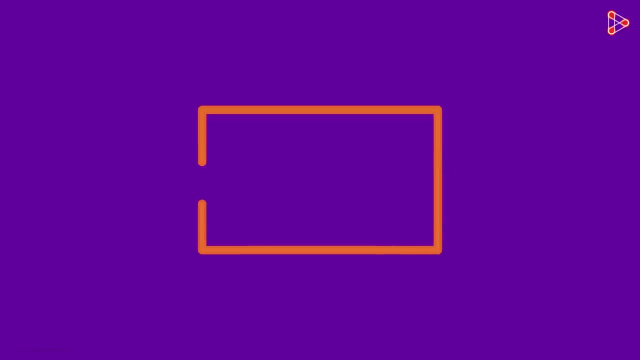 We'll come to that factor soon, don't worry. So if we just have a copper wire, do you think electricity will flow through it? Clearly not, because there's nothing that's triggering it. There's no factor triggering it. So what is the factor that triggers the flow of electricity? 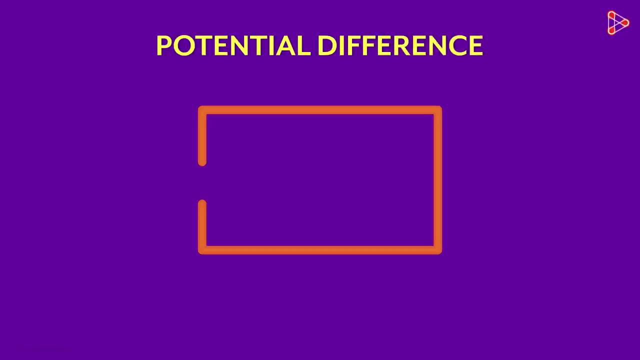 It's called the potential potential difference. Now, I can't define this term in one line, but that wouldn't help you understand the concept well, So let's dive a bit deeper into it. We see the word potential here. Have you heard this term before? Of course we've heard. 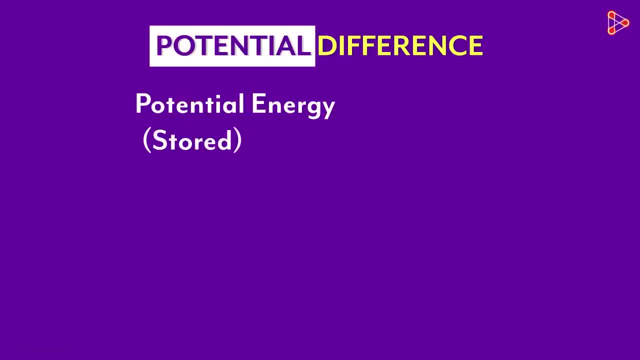 of potential energy. It is the stored energy. when an object is at rest, When you're holding a ball in your hand, it has potential energy. When you drop it, the potential energy is getting converted to kinetic energy. when it drops to the ground, Kinetic energy is the energy an object has when it's in. 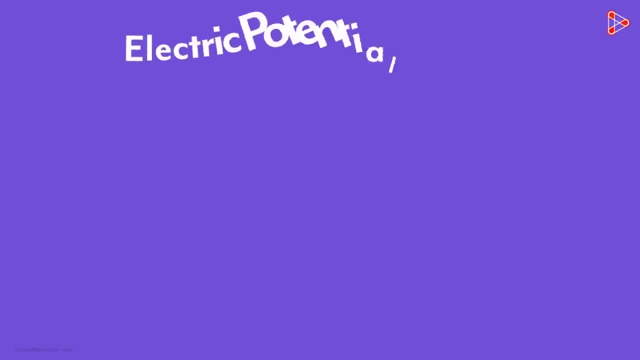 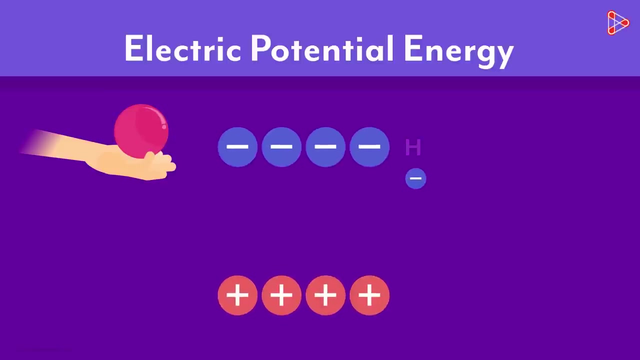 motion. Similarly, there is a concept of electric potential energy. The electric potential energy of any charge describes how much stored energy it has. Just like the ball in your hand has high potential energy. a negative charge close to another negative charge has high potential energy If left free the charge. 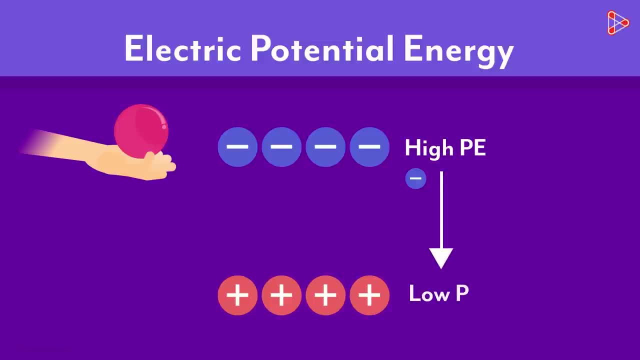 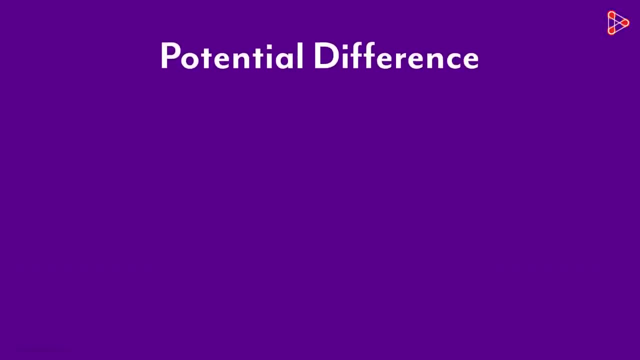 will be repelled by the negative charge and will move towards the positive charge, Just like the ball will fall towards the earth. What's potential difference then? It's just a difference of electric pressure between two points, And this difference may arise because of a battery consisting of cells. Potential: 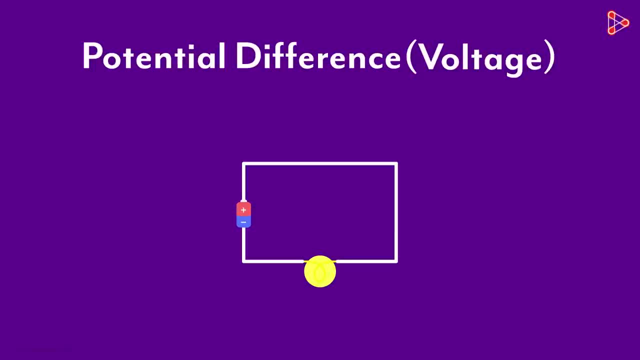 difference is also referred to as voltage. If we have to understand the technical definition, we would say that it is the work done to move a unit charge from one point to another. The potential difference V between any two points in an electric circuit will be: 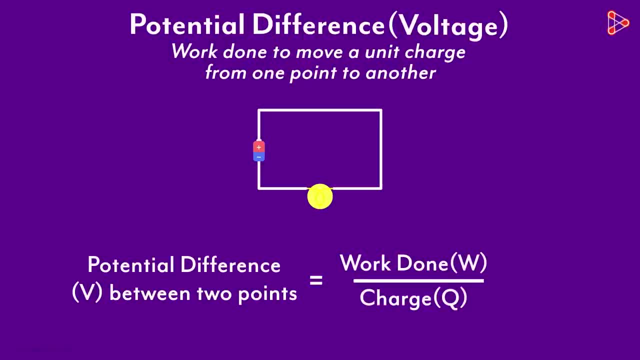 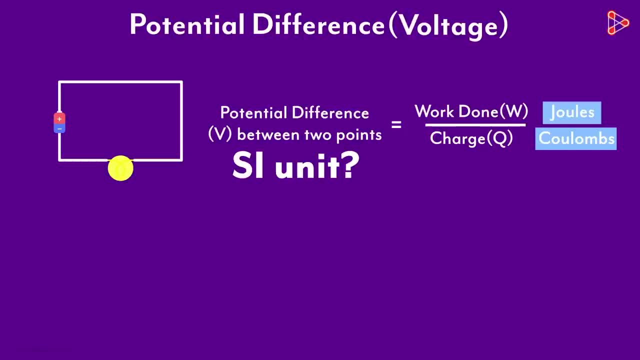 the work done over the charge Q. We know that the work is measured in Joules and charge is measured in Coulombs. What's the SI unit of potential difference then? It's Volt, named after Alessandro Volta, an Italian physicist. So how would we?